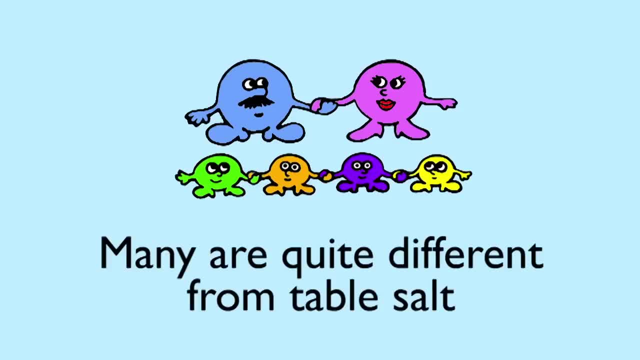 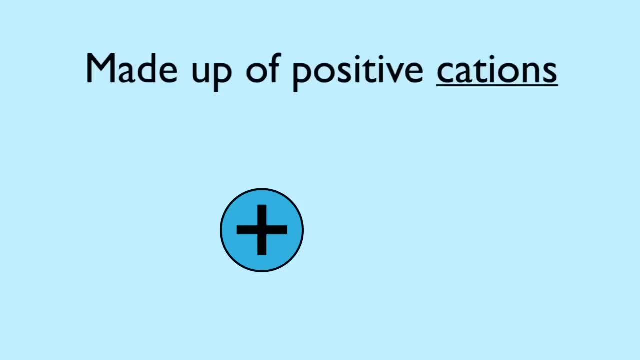 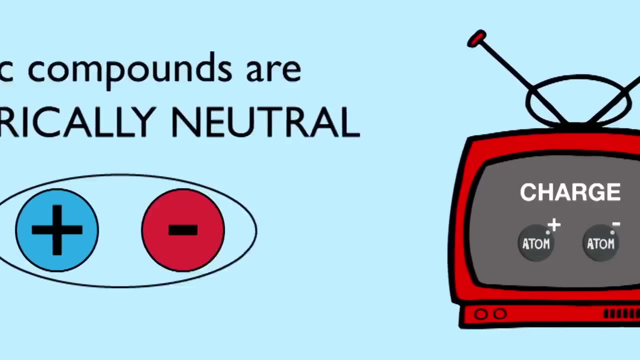 different properties and uses to table salt. Let's start with what a salt is. It's an ionic compound made up of one or more positively charged cations and negatively charged anions. An ionic compound is electrically neutral. Watch this video if you'd like a refresher on this. 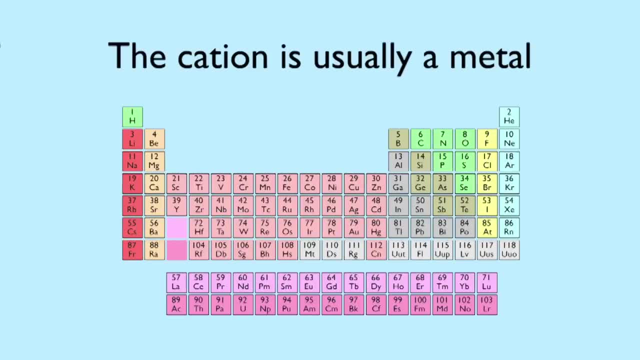 concept. A cation tends to be a metal and in many common examples is one from group 1 or 2 of the periodic table. The anion is commonly a halide from group 7 or a member of group 6.. Salts made. 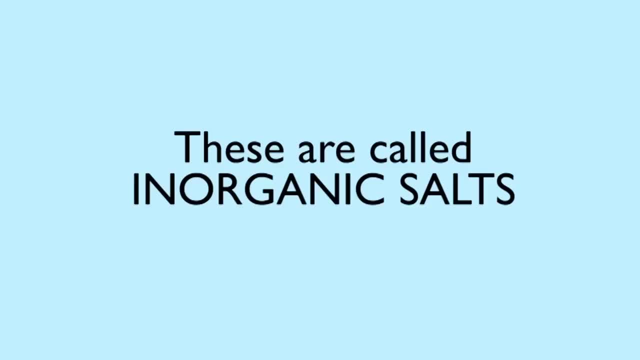 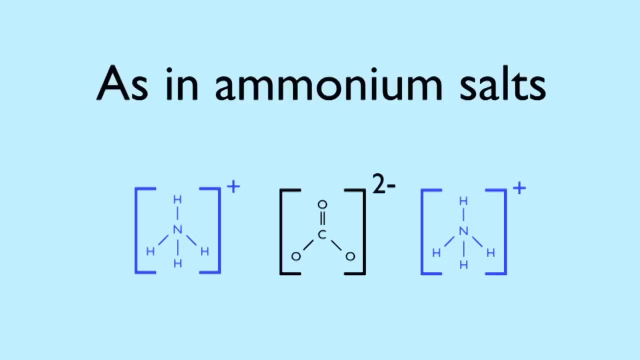 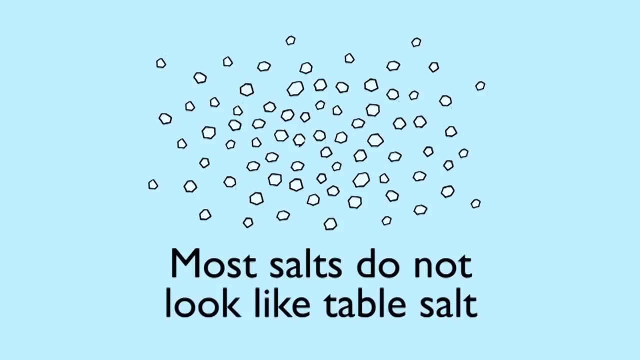 like this are called inorganic salts, but this is not always the case. The ions can be polyatomic, that is, made up of more than one atom. A common example of this would be ammonium salts. You might wonder if all salts are small, transparent crystals, just like table salt. Certainly not. 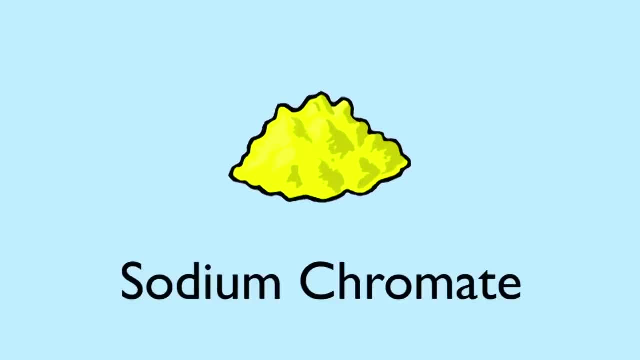 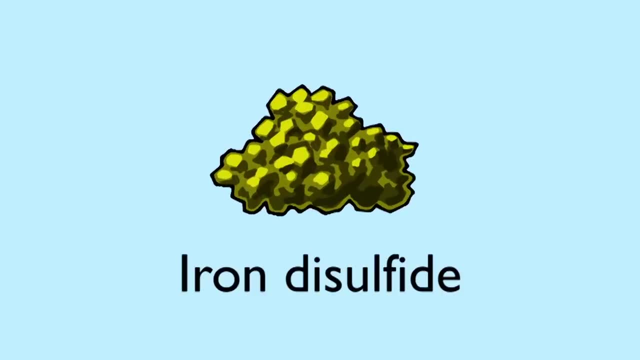 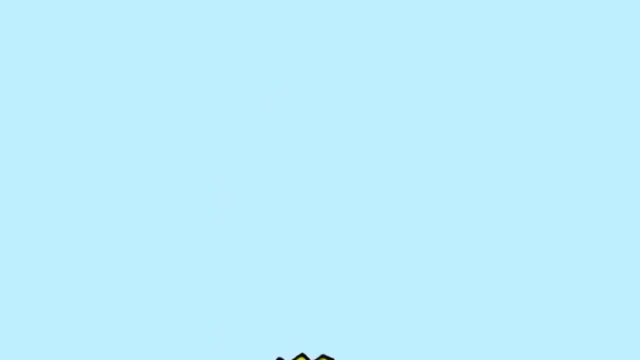 Salts come in many different colours. Sodium chromate is yellow, potassium permanganate is purple and iron disulfide is shiny and metallic. In fact, it's a mineral commonly called fool's gold. Another common mistake is to think that all salts taste well salty. Again, this is wrong. 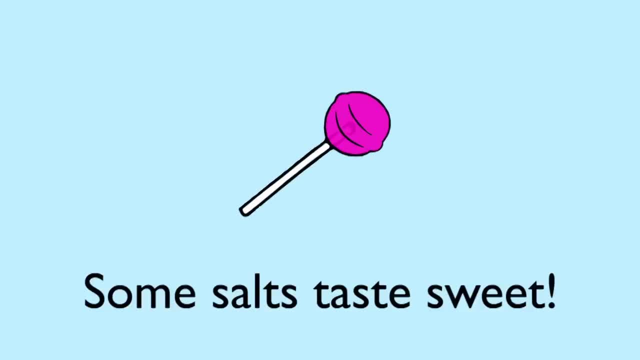 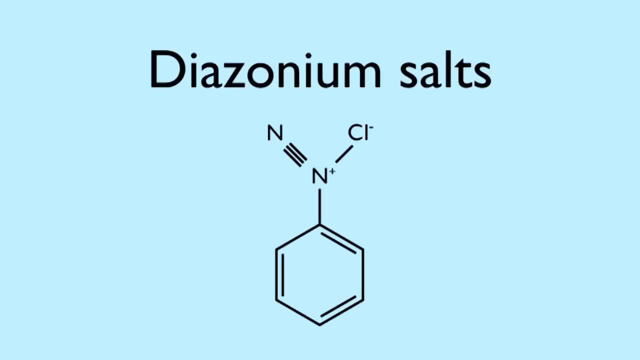 Some taste bitter and some even taste sweet, like lead diacetate. Unfortunately, it's also poisonous. Here's another more complicated salt with nitrogen in the cation. It's part of a family called the diazonium salts, which are all brightly coloured. Can you think what they might be used for? 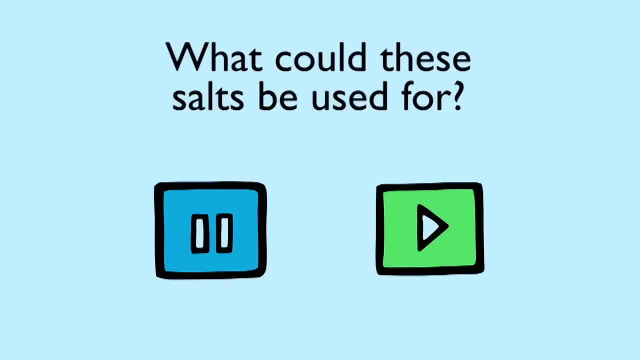 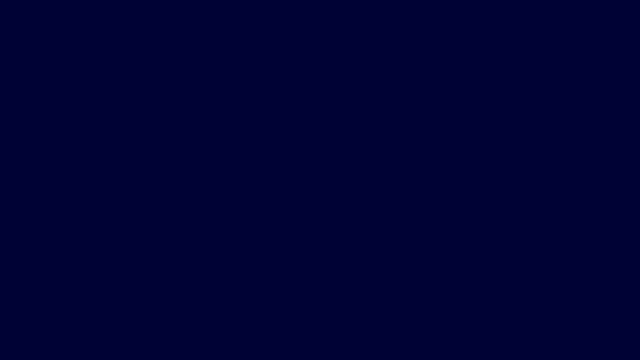 Pause and have a think, then resume. The answer is: they're used for dye pigments to colour our clothes. If you ever get the chance to see a salt, please do so. If you ever get the chance to enjoy some fireworks, the bright colours you can see are produced by 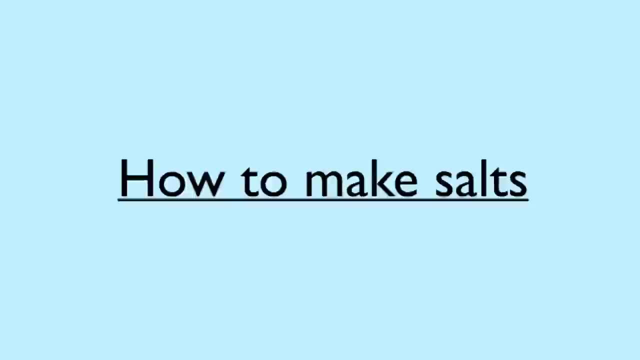 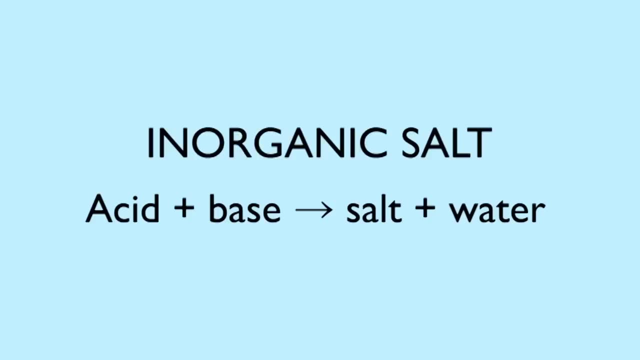 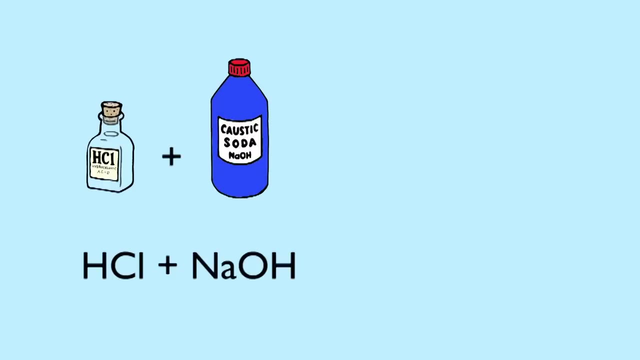 burning the salts of various metals. You might recall learning that an acid plus a base gives you a salt and water, and that's quite right for an inorganic salt. Here's the classic reaction for making sodium chloride. Hydrochloric acid plus sodium hydroxide equals sodium chloride and water. 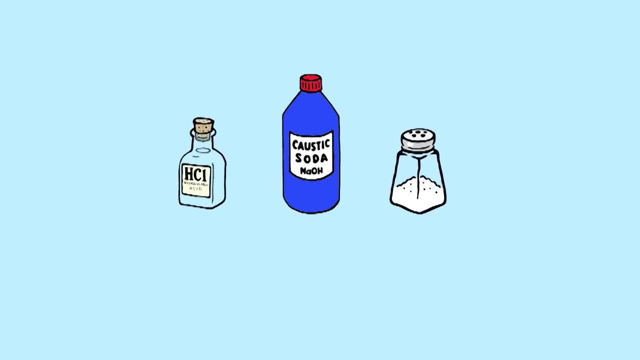 Here's the thing, though: Hydrochloric acid, sodium hydroxide and water are both salt and water. Hydrochloric acid, sodium hydroxide and sodium chloride are all water-soluble and dissolve to form clear solutions. So the challenge is: can you think how you would monitor this reaction?